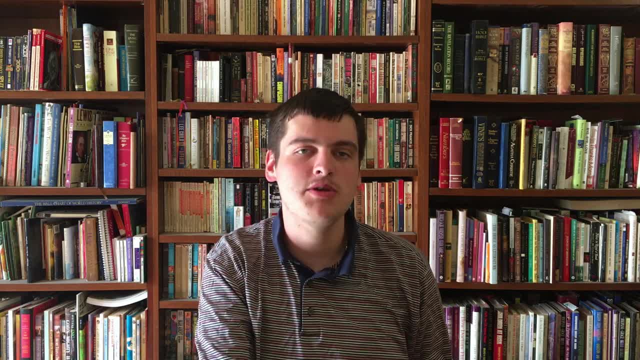 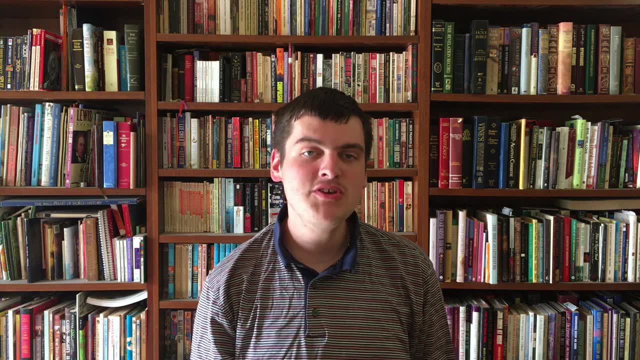 Math is a scary word. It's the worthless formulas that we pretend to understand but have no real value or relevance in the world, Or that's what many people are led to believe. But if you stop looking at algebra as just the thing you need to do to pass high school, 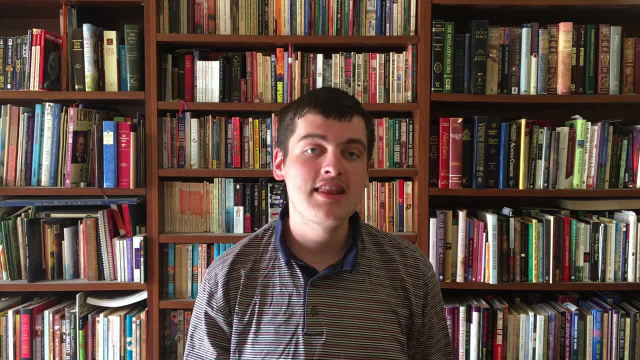 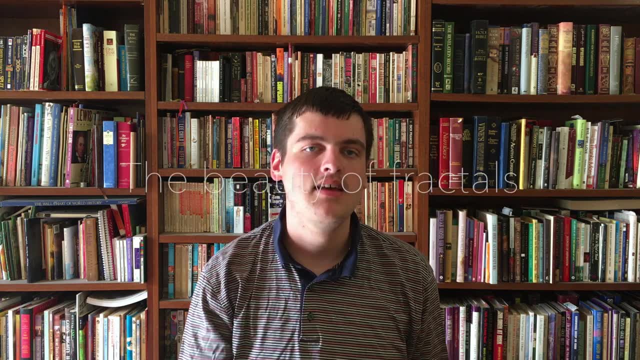 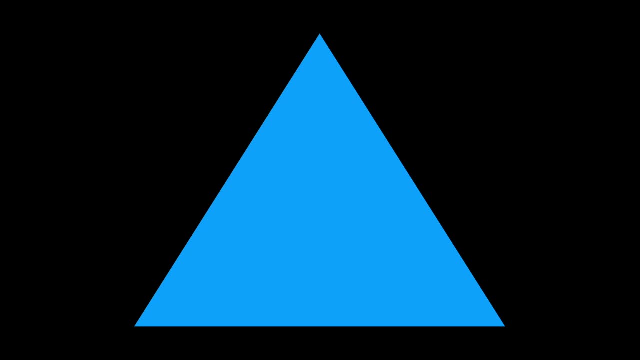 you can see many parts of it that are beautiful, practical and the basics for laws of the entire universe. One great example of all these things is fractals. So what is a fractal? Well, imagine for a moment we had a triangle like this: 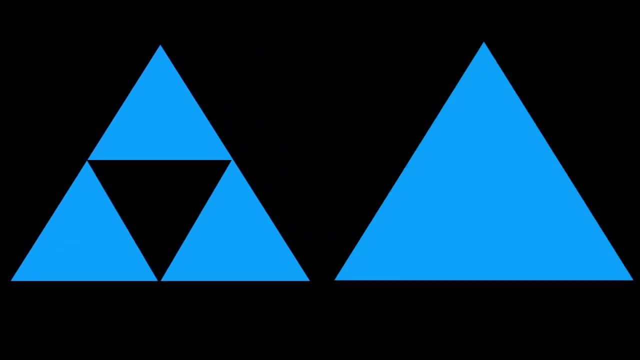 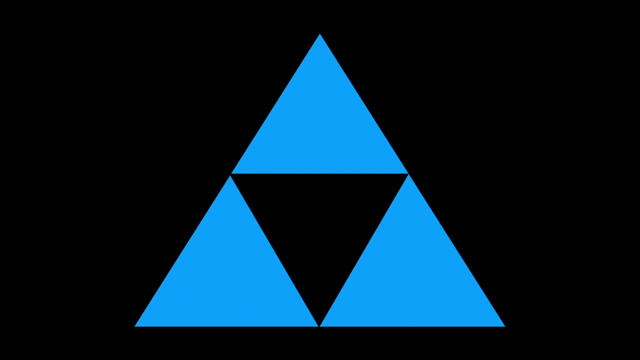 and we cut out the center of it like this. Now you'll notice that each part of this shape is the same as the original shape we had before. We can continue to do this to each of the new triangles, each time getting a shape that is identical to the original shape we had. 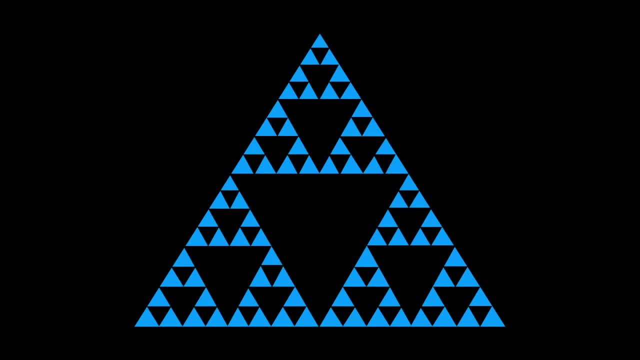 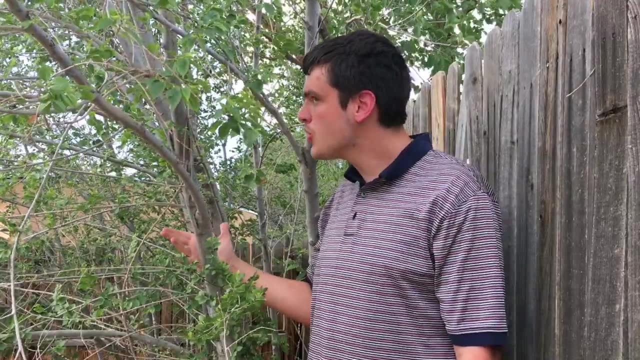 This is the defining trait of fractals: self-similarity. Now, you've probably seen this sort of thing before. Take, for example, this tree. We got the trunk- we can call that the original shape- and then we have these branches, But the branches. 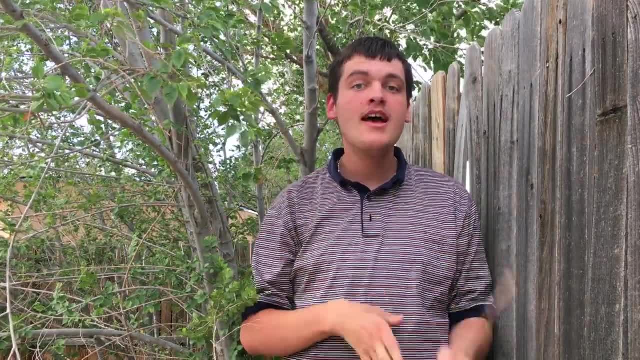 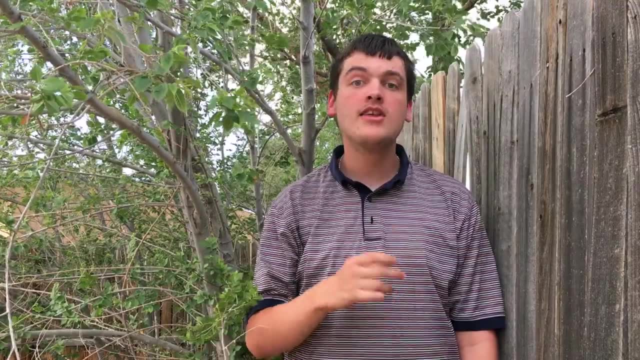 are simply just the same shape, just getting smaller and smaller. This sort of self-similarity is incredibly common. Fractals are a pattern in tons of art and it's really funky stuff. There are variations of plants that are fractals. Lightning stripes are fractals. 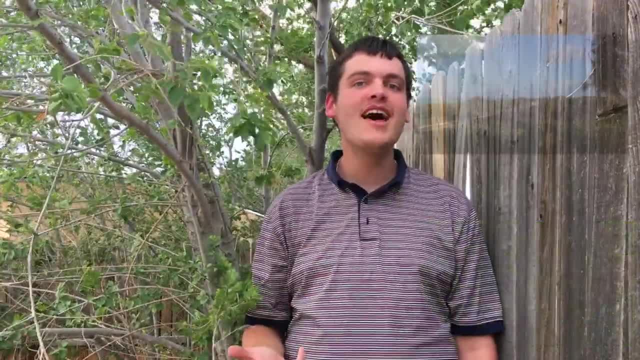 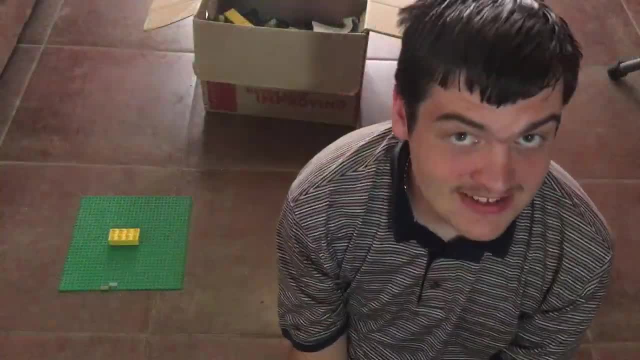 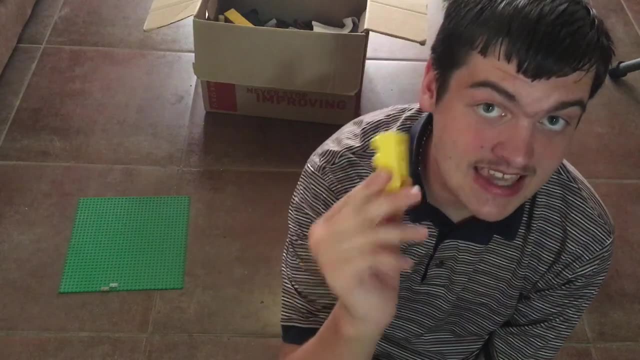 Everything from flowers to vegetables to coastlines and even universes All follow this pattern of self-similarity. A good, practical use of fractals is their surface area. It can be difficult to wrap your head around, so let's pretend that each of these Legos is a capillary. 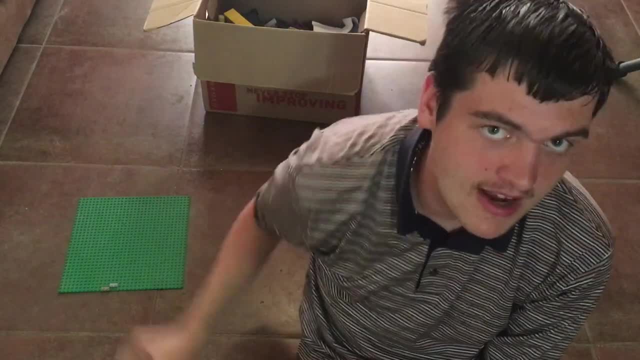 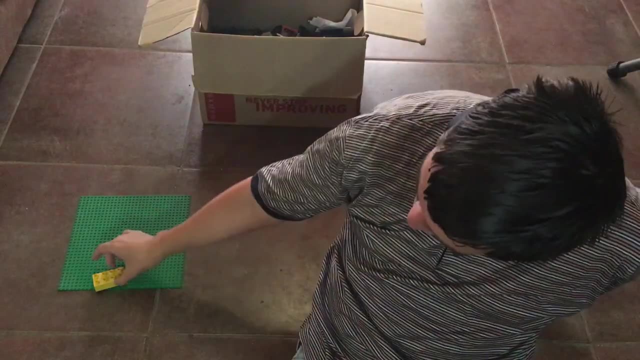 the tubes that transport blood and oxygen to the various parts of your body. Now the human body needs about 10 billion of these, and we need to fit them all inside this space. How are we going to do this? As useful as this big shape is, if I just start placing these? 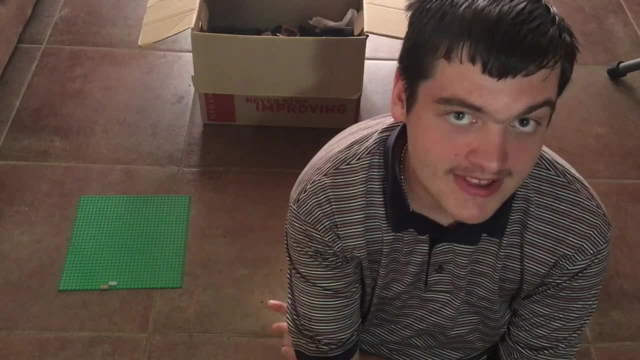 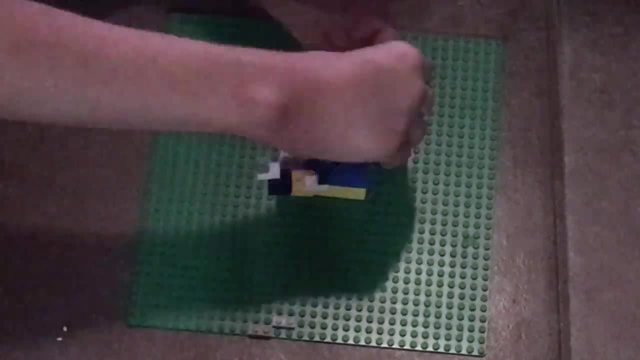 I'll be able to move around the room quickly. So obviously I should place some smaller Legos and then eventually even smaller Legos, And as long as I can continue to keep this shape, I can place these over and over again forever. This is how the human body can fit billions of.